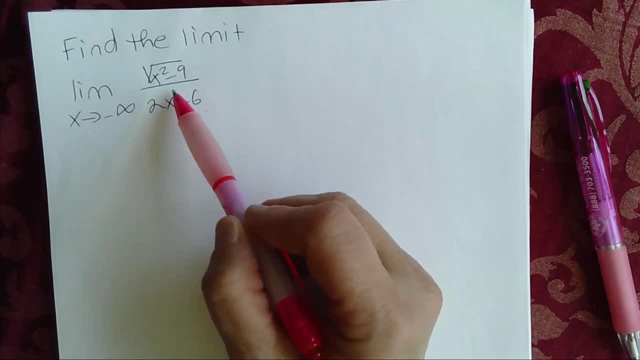 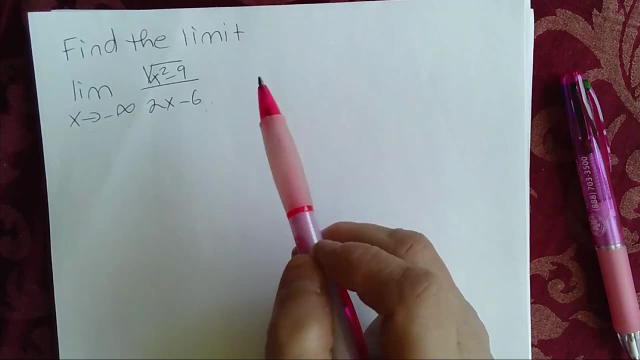 And in this case the variable with the highest power is x. that's the only variable in the denominator. So what you've done in the past is that you divided both the numerator and the denominator by x. But here you have to be careful, because you have a square root. 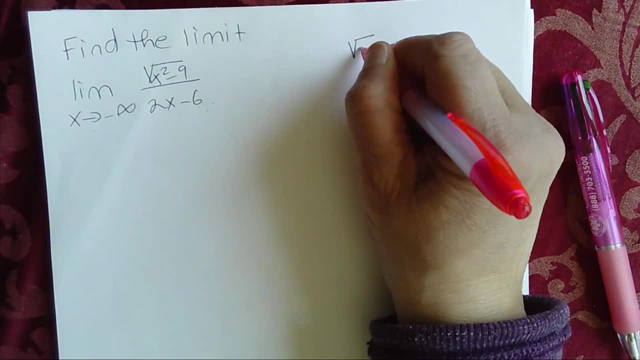 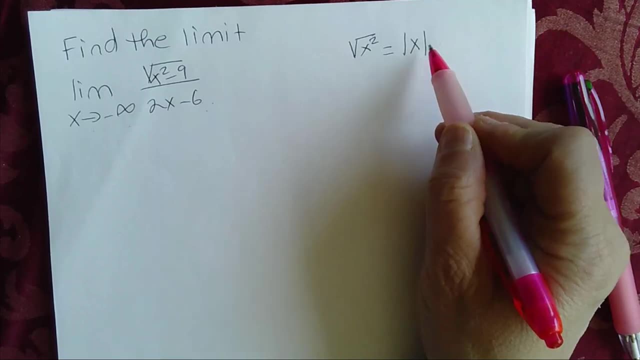 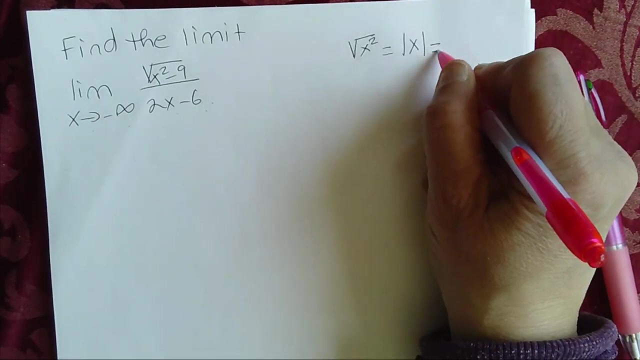 Now, to remind you, square root of x, squared from algebra, is equal to absolute value of x. Now, this is equal to x if x is positive, But in this case x is negative. x approaches negative infinity, So this is equal to negative x again because x is negative. So what we? 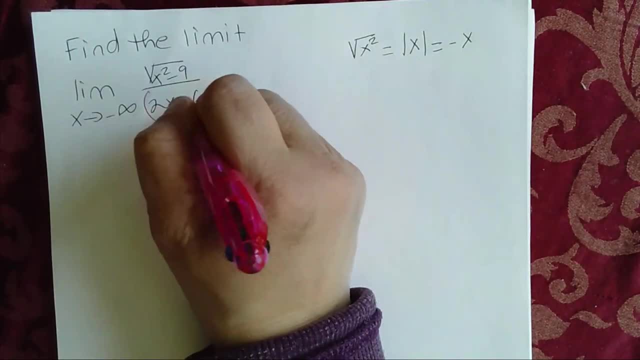 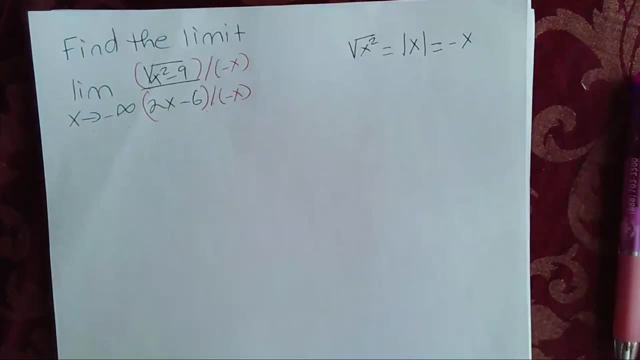 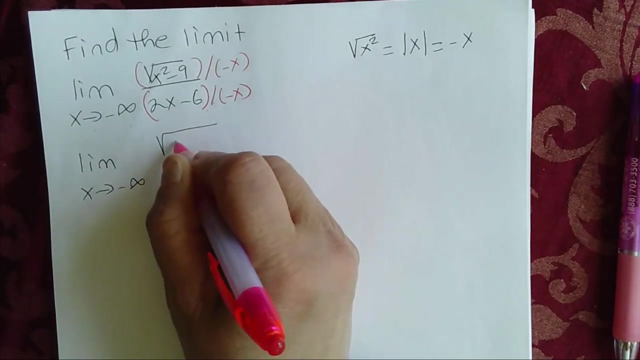 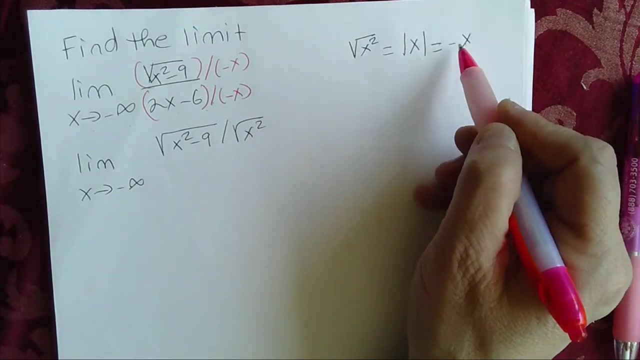 have to do here is we have to divide both the numerator and the denominator by negative x. Now this will give me, in the numerator, the square root of x squared minus 9 divided by square root of x squared. Remember, this is equal to this: You have 2x divided by negative. 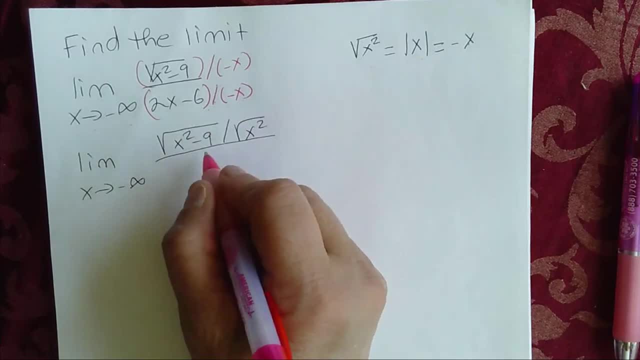 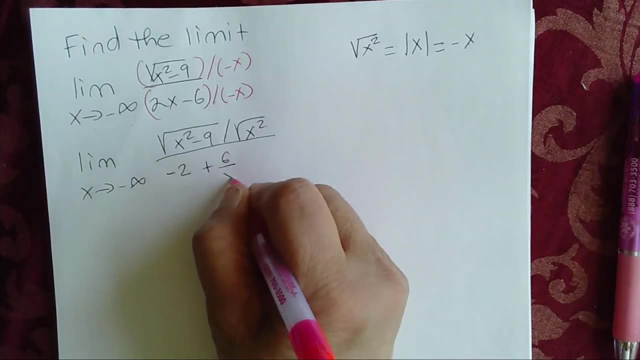 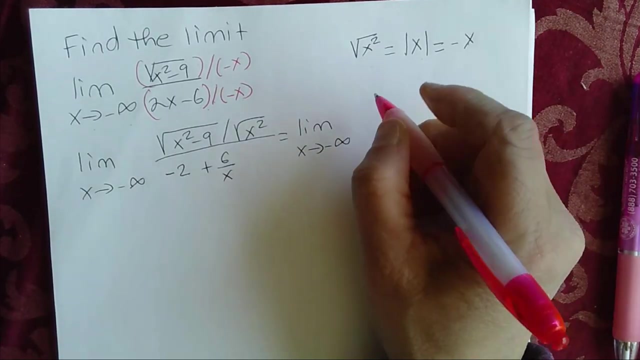 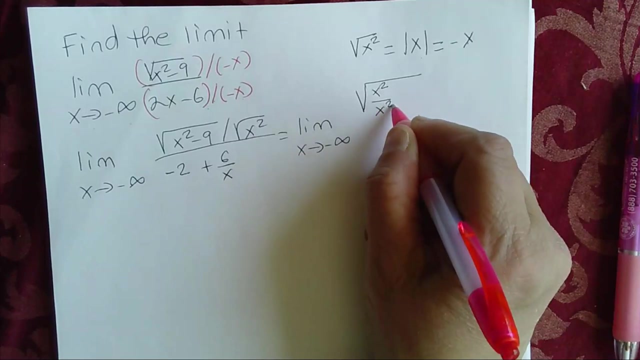 x, that will give me negative 2.. Negative 6 divided by negative x, that will be positive 6 over x. Let's go ahead and simplify the numerator: The limit as x approaches negative infinity of x squared divided by x squared minus 9 over x squared divided by negative 2 plus. 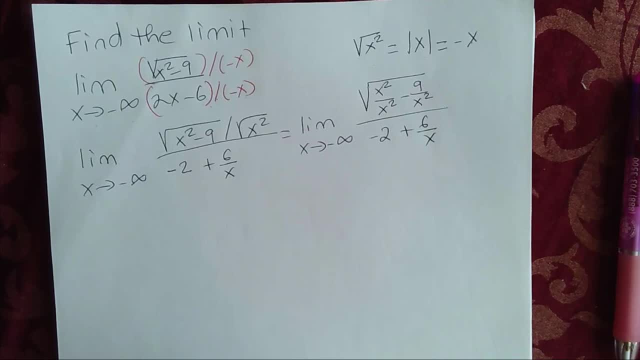 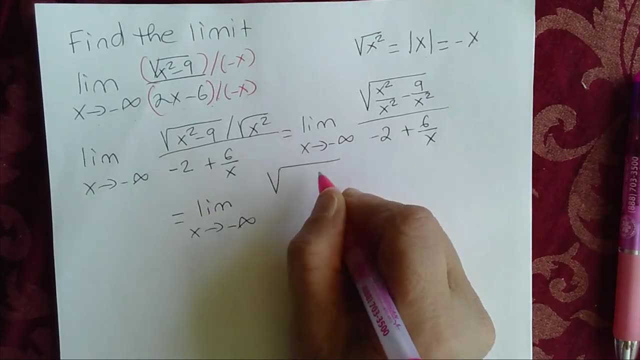 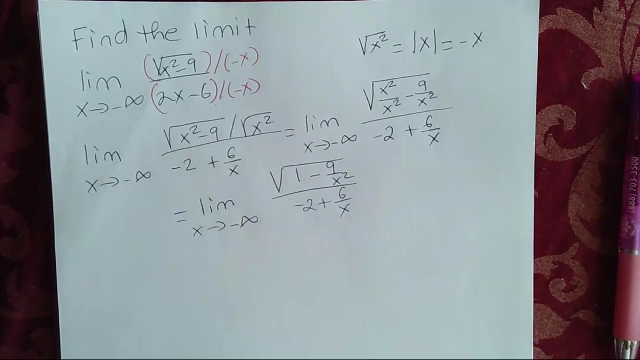 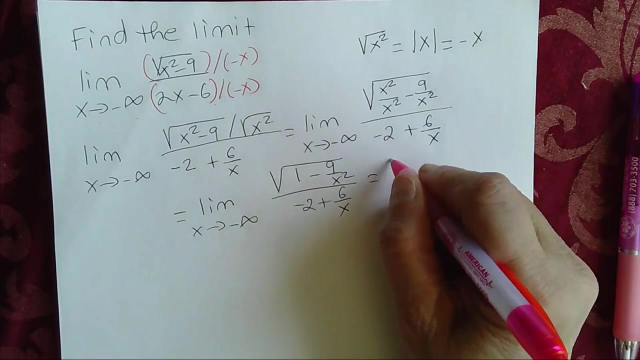 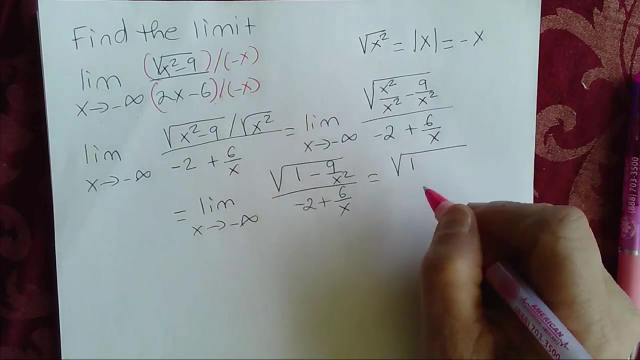 6 over x, Simplifying the numerator. then we get the limit as x approaches negative infinity of square root of 1 minus 9.. Now we can apply the limit laws, The limit of 1 as x approaches negative infinity, remember that's a 1.. The limit of a constant as x approaches anything is simply the constant minus the. 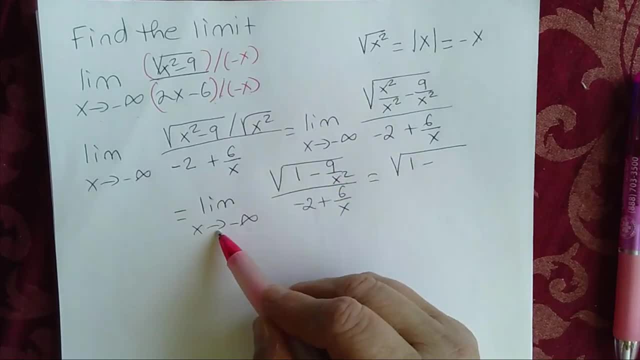 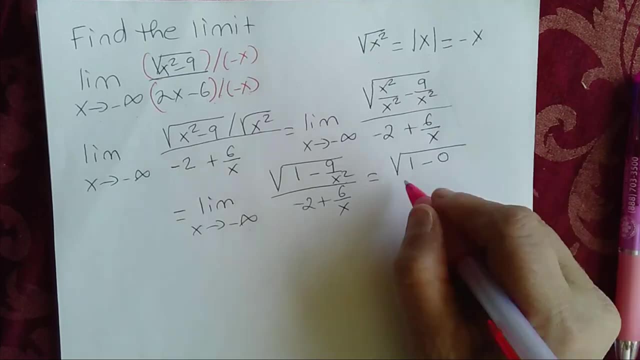 limit of 9 over x squared as x approaches negative infinity, that's going to be 0.. This is going to approach 0 as x approaches negative infinity. In the denominator you have the limit of negative 2, it's simply negative 2, plus the